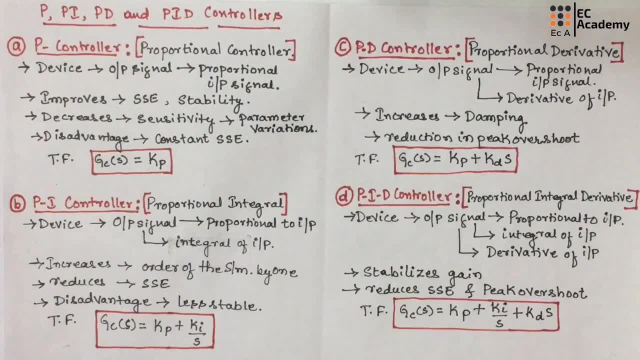 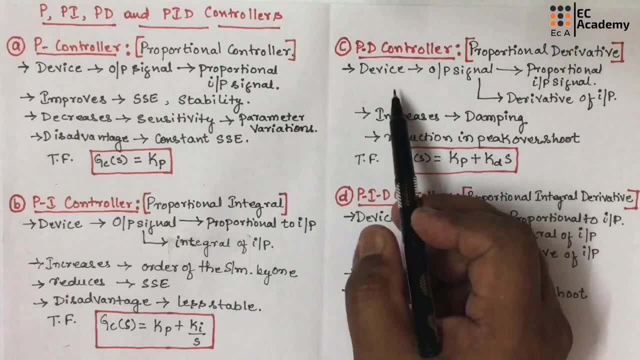 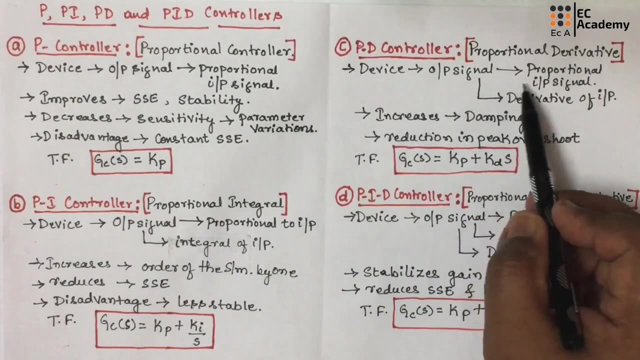 are representing the transfer function in terms of Laplace domain. Next type of controller is PD controller, which is proportional derivative controller. The proportional derivative controller is a device that produces an output That consisting of two terms: one is proportional to the input signal and other is proportional. 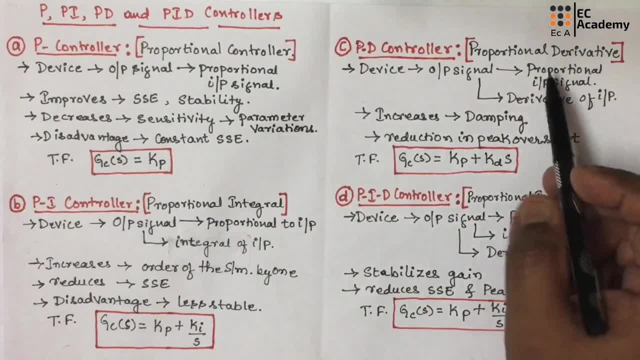 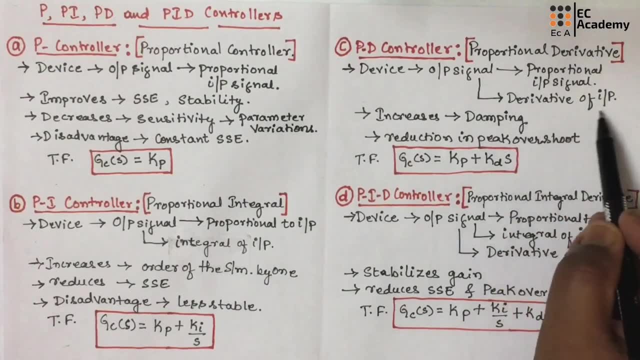 to derivative of the input signal. So it will produce the output, which will be having two terms. First term is the output is directly proportional to the input, as well as the output will be the derivative of the input. Such type of controller are known as PD controller. 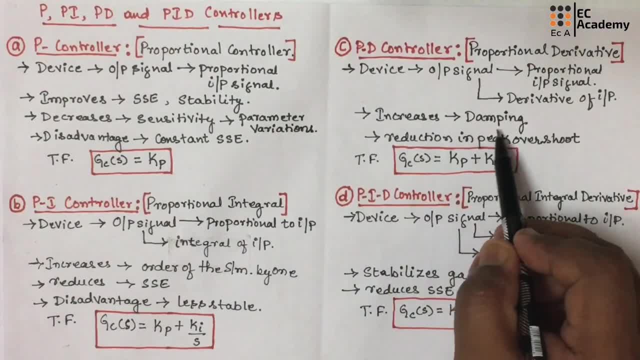 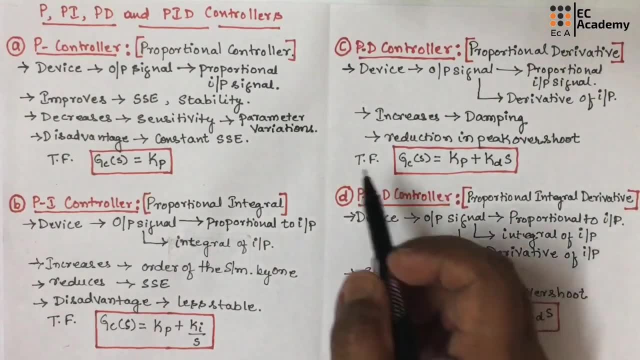 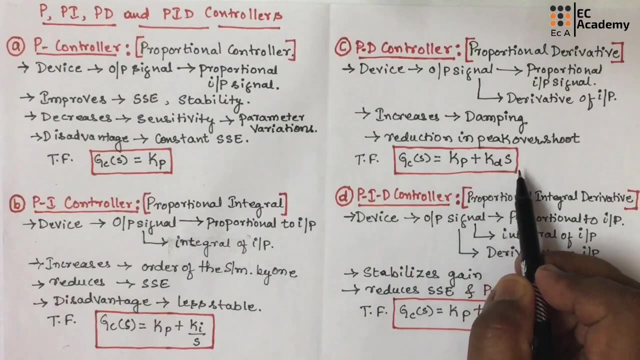 The effect of PD controller on the system performance is it will increase the damping ratio Of the system and also there is a reduction in peak overshoot. The transfer function of PD controller is given as gc of s is equal to kp plus kd s. 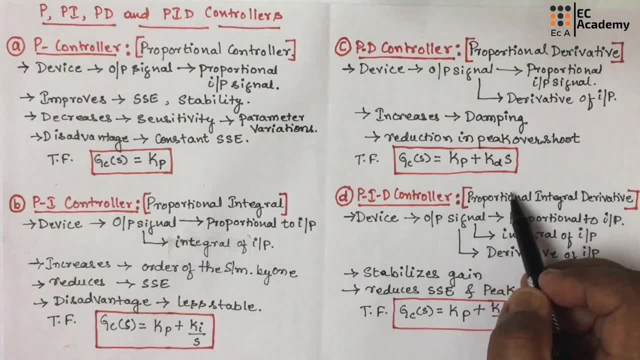 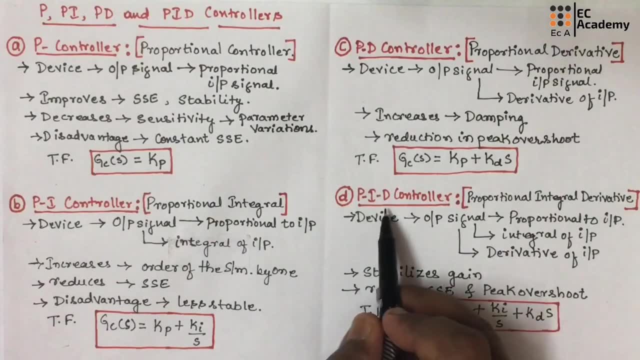 So here the term kd represents derivative constant, kp is the proportionality constant. The next type of controller is PID controller, which is proportional, integral derivative. It is a device that produces an output that consisting of three terms. First, one is proportional to the input signal. 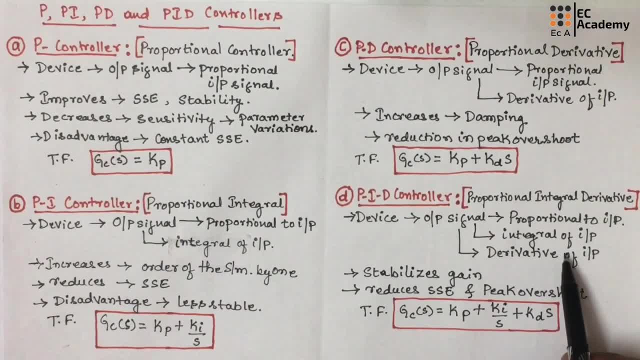 Another one is proportional to the integral of the input signal and the third one is proportional to the derivative of the input signal. The PID controller stabilizes the gain, reduces the steady state error and also it reduces the peak overshoot. The transfer function of PID controller is given as gc of s is equal to kp plus kd s. 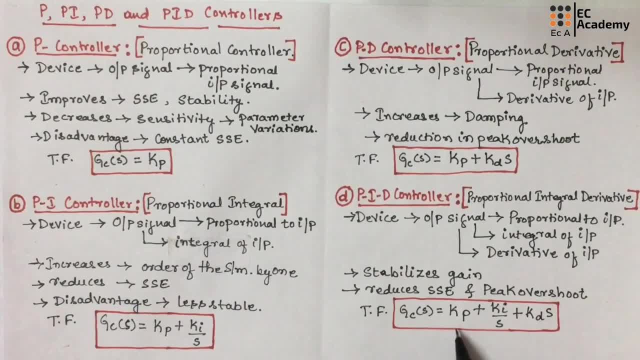 The transfer function of PD controller is given, as gc of s is equal to kp plus kd s. The transfer function of PD controller is given, as gc of s is equal to kp plus kd s. So here kp is the proportionality constant, ki is the integral constant and kd is the.